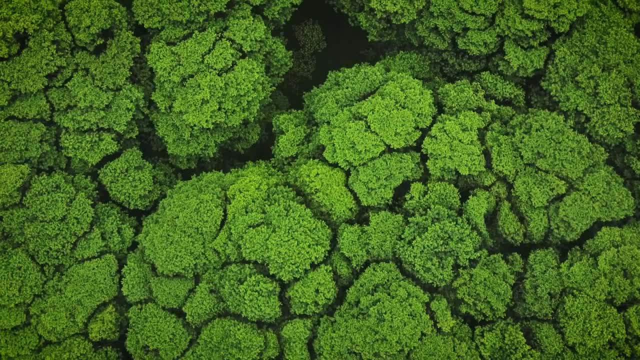 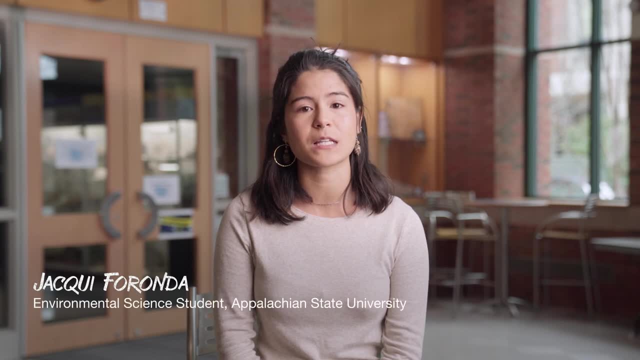 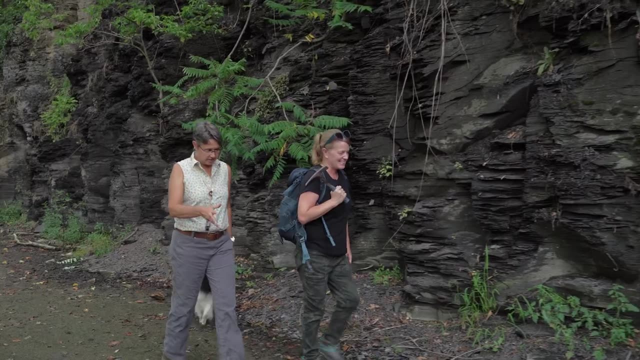 ocean and climate conditions above the water changed this event and connect these to changes in reef communities. By reconstructing what conditions were like leading up to and through this extinction event, we can better understand how our modern reef ecosystems might react to changes in the environment. 365 million years ago, there were many areas in the world's oceans. 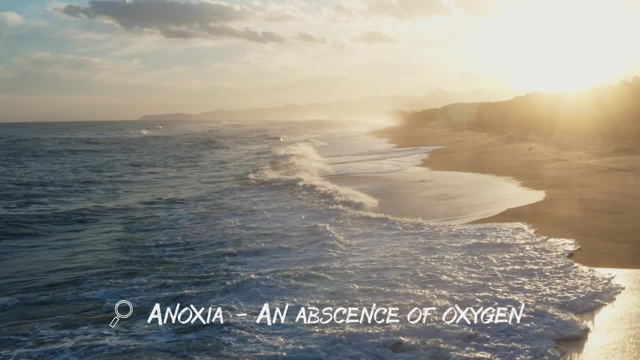 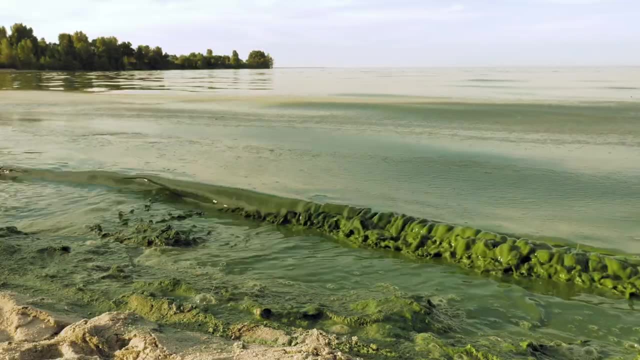 that were anoxic or had severely reduced oxygen levels. While we do not see these conditions in our oceans today on the scale that they occurred in the Devonian, we are seeing an increase in anoxia in coastal waters. These conditions in modern environments are often associated with: 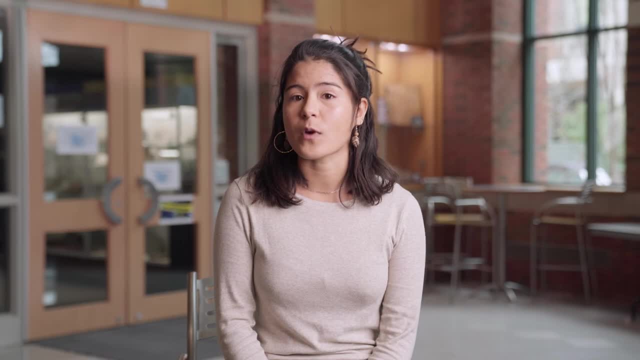 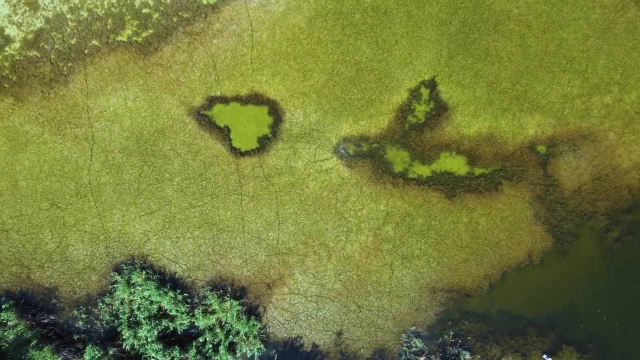 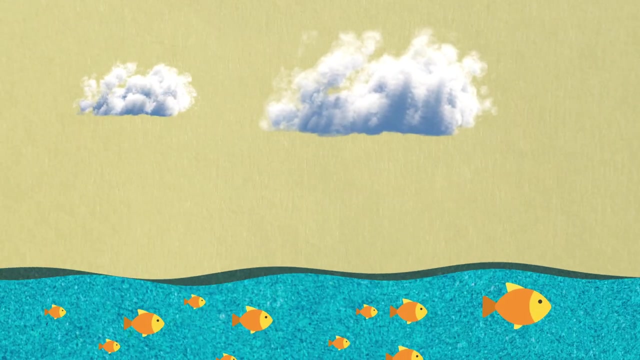 increased nutrients dumped into the oceans. Nutrient-dense runoff can be sourced from agriculture, sewage or other manmade waste. This influence of nutrients, or essentially food, results in an explosion of algae in the surface waters. This dramatic increase in the amount of algae has a number of negative 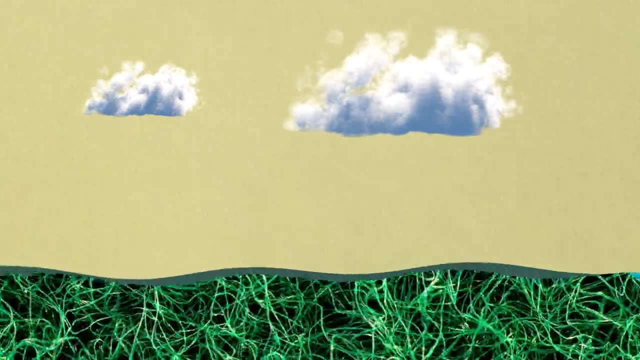 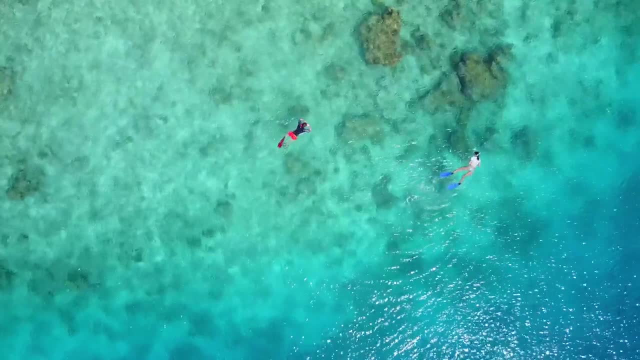 effects. The algae uses up all of the available oxygen in the water and it impacts all marine life in the immediate area, causing anoxia. Coral reefs are incredibly sensitive systems. In order to thrive, their environment must be relatively stable and resilient. 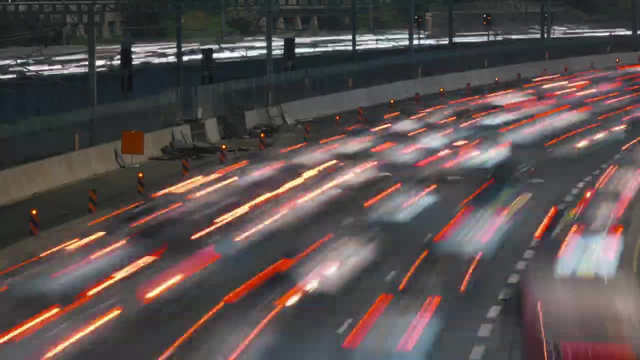 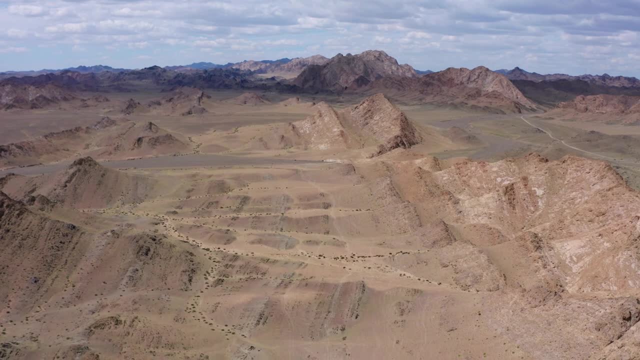 By studying the environmental stressors of today, we have a bit more insight of what would have led to the demise of coral reefs of the past. What caused the late Devonian mass extinction? We don't know for sure, which I think is really. 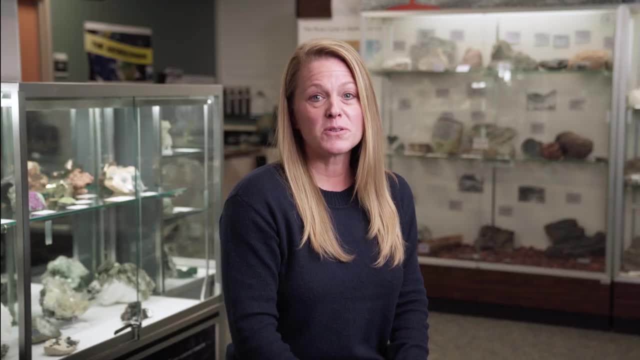 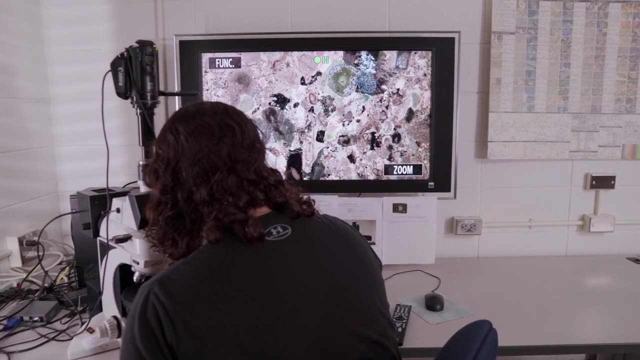 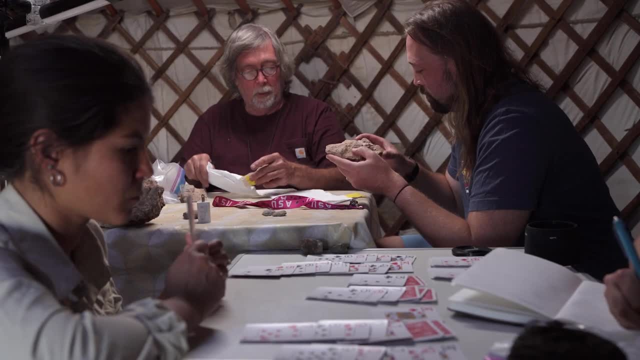 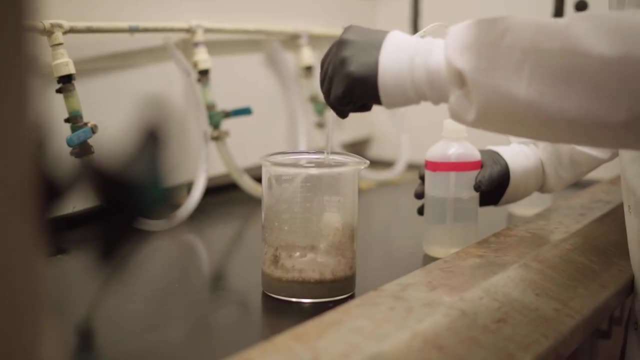 in convertible oceans 365 million years ago, using patterns in the layers of the rocks, hand samples and even signals preserved at the atomic scale. hand samples and even signals preserved at the atomic scale. We need to look at the evidence collected from different environments, and this can take us all around the world.